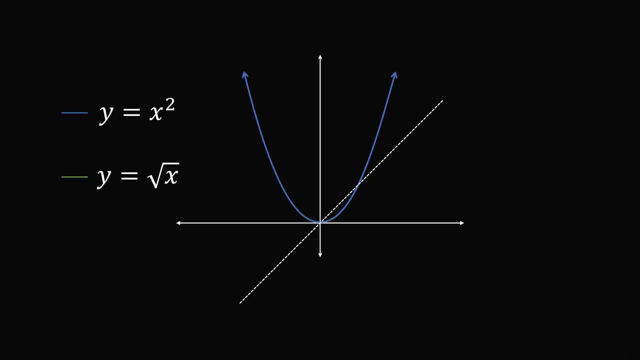 You can invert functions by reflecting them about. the line y is equal to x, So we would end up with this parabola. Now we have a problem with this parabola. This is not a problem. This is not going to be a function. 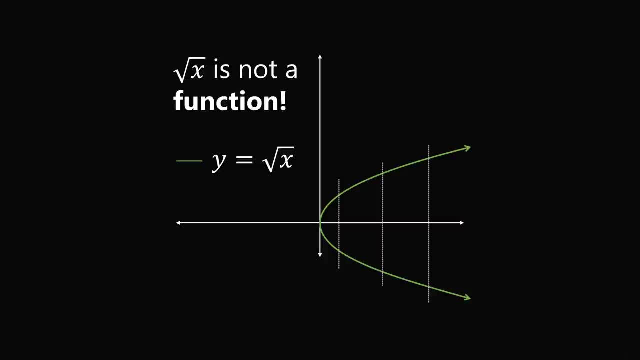 By the vertical line test, we can see that every single x value greater than 0 is being assigned to two y values. A function has to assign every single x value to one y value. So how can we fix this? Consider a tree with many different branches. 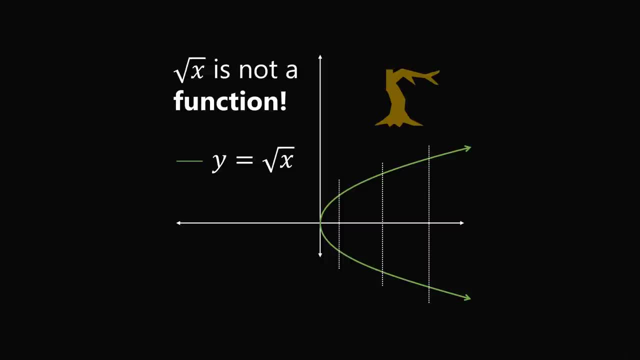 You could prune off some of the branches, so you're left with just one branch. So we're going to do the same thing here. This parabola has two branches, one going up and one going down. So if we prune this bottom branch, we're left with just one branch at the top. 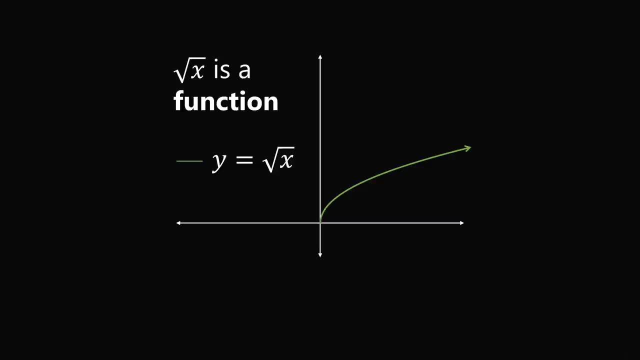 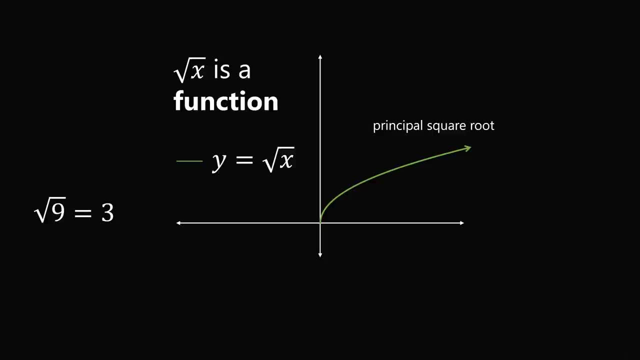 So square root of x is a function. So square root of x is a function. So square root of x is a function. So square root of x is equal to 3, which is 1 value. So, to summarize, if x is a positive number and n is a positive integer, 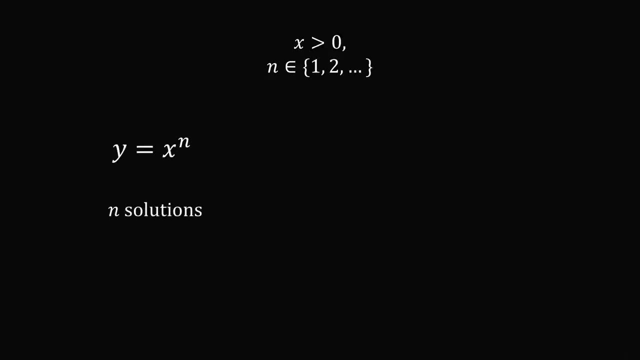 we have, y is equal to x to the power of n. This will have n solutions. If we take the nth root of x, this will exactly be equal to x to the power of 1 over n, And this will be the principal root. 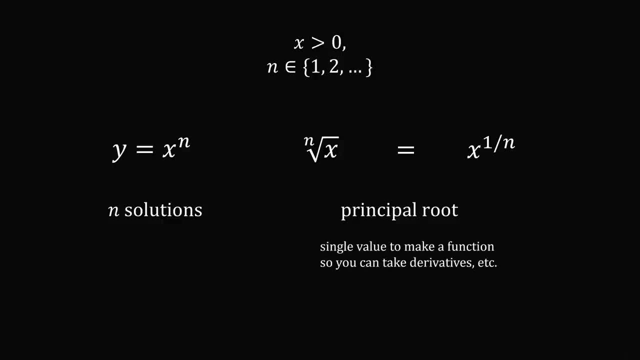 And again, we take a single value so that we can make a function, so we can do everything we could normally do with functions. Now what if, instead, we consider: x is less than 0? y is equal to x to the power of n. 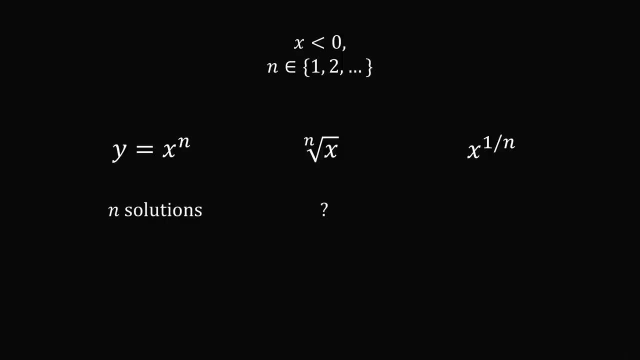 We'll still have n solutions. But what can we say about the nth root of x and x to the power of 1 over n? In order to understand that, we have to get complex. So we have the complex plane here and consider a number: z is equal to a plus bi. 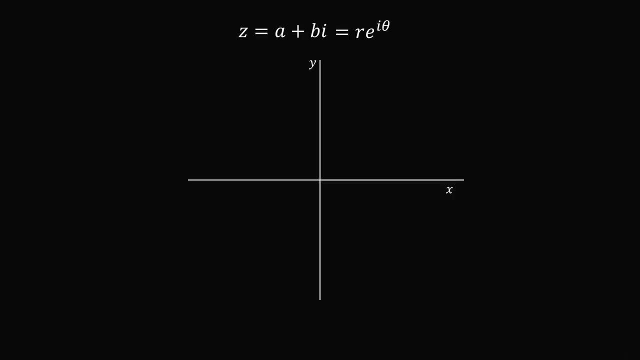 We can write this in polar form as r multiplied by e to the i theta. So imagine we have a circle here We have the point z, So the radius of this circle will be r, and then this angle theta will be theta. 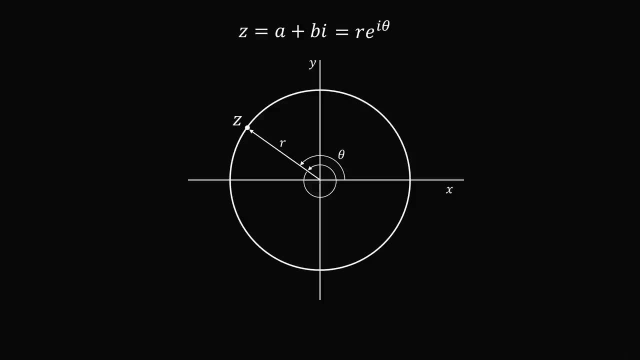 Now, of course, you could add any multiple of 2 pi. You'll still get the same angle. So we could also write this as r multiplied by e to the power of i multiplied by the angle theta plus 2 pi k, where k is an integer. 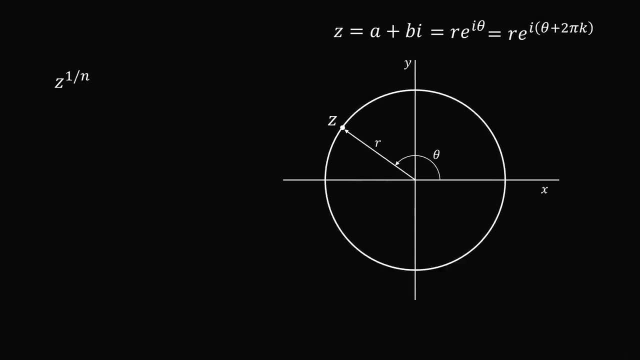 So now we want to take z to the power of 1 over n. This will be the set of n roots. Now we can do this to the polar form and we get the result: the nth root of r multiplied by e to the power of i, multiplied by the angle, theta over n, plus 2 pi k over n. 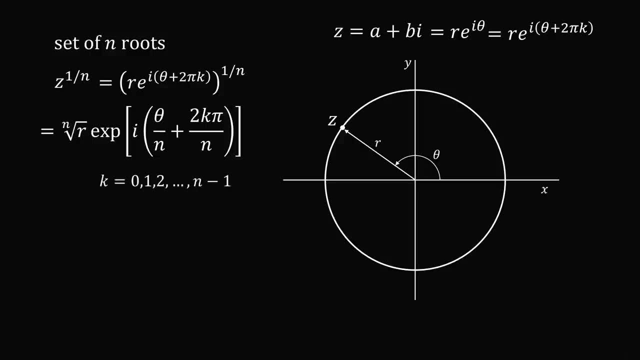 This will have distinct roots for k equaling 0,, 1,, 2,, all the way to n minus 1.. The n roots also have a nice graphical interpretation. They will be the nth root of 1 over n, So we'll write this as z to the power of 1 over n. 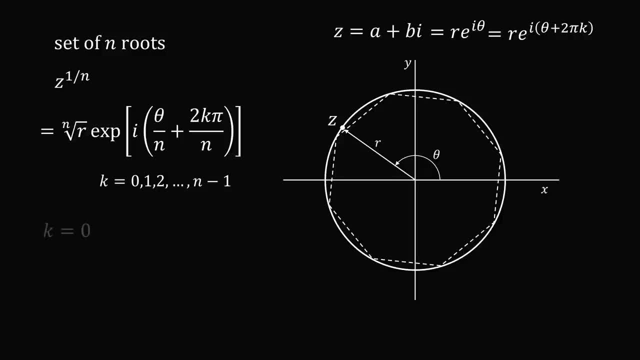 This will be the set of n points of a regular n-gon. Now, if you set k is equal to 0, you get the principal value of the nth root of z. So let's see how this works out with. z is equal to negative 1.. 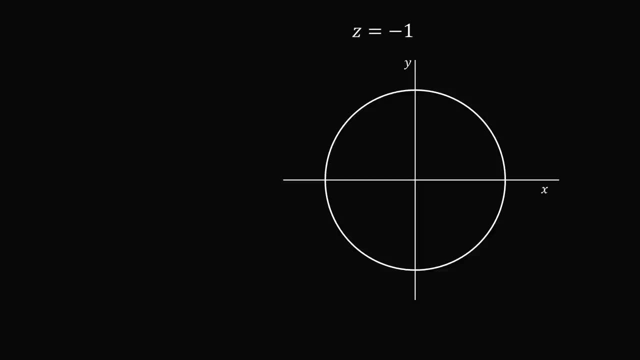 So first we have: z is equal to negative 1.. We want to write this in polar form. So we first see that z is equal to negative 1. is this point right? here? The radius will be equal to 1, and the angle will be: theta is equal to pi. 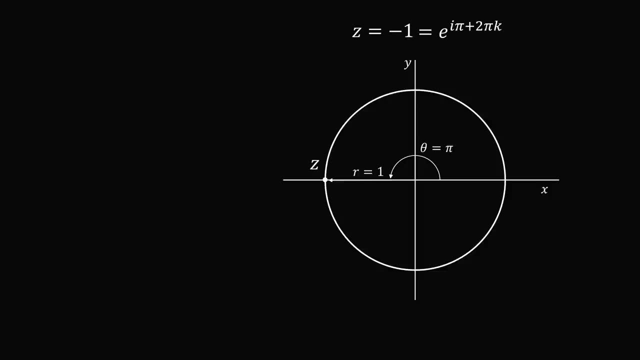 So in polar form we have: z is equal to negative 1.. This is equal to e to the power of i pi plus 2 pi k. We now want z to the power of 1 over 3.. So this will be the set of three roots. 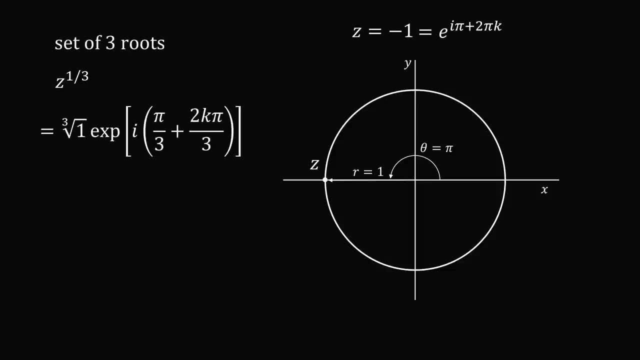 This works out to be the cube root of 1 multiplied by e, to the power of i multiplied by the angle pi over 3, plus 2, pi k over 3.. We get distinct roots, for k is equal to 0,, 1, and 2.. 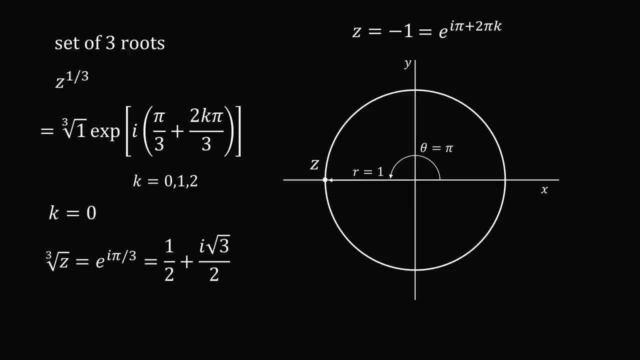 So we set k is equal to 0. We get the principal root, which is e to the power of i pi. So we have e to the power of i pi over 3, which equals 1 half plus i root, 3 over 2.. 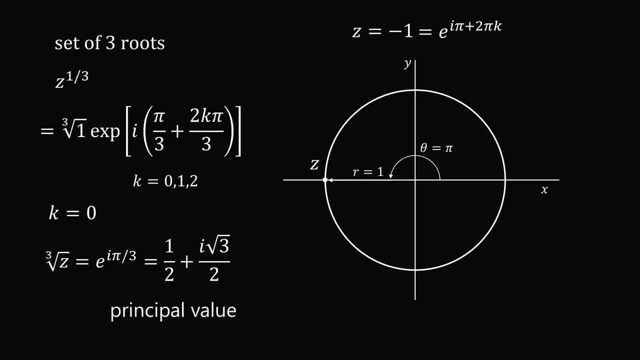 And this is exactly what WolframAlpha was outputting as the principal value of negative 1 to the power of 1 over 3.. If we plot the three roots, we get that they are the endpoints of this equilateral triangle. We have the principal value here, then we have the real root of negative 1 comma 0,. 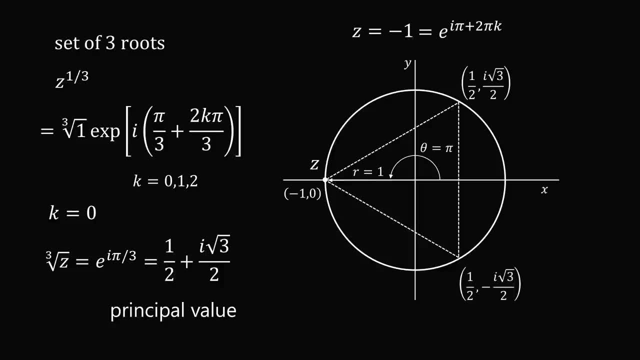 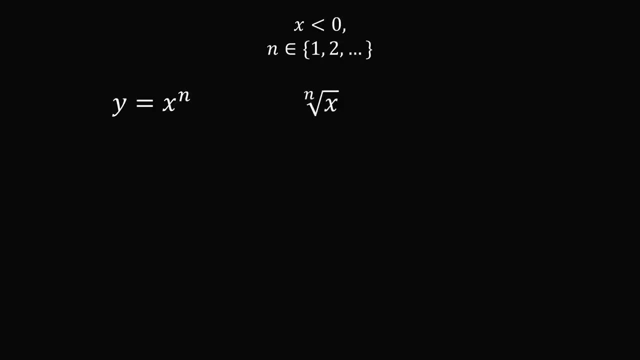 and then the other root is the conjugate of this principal root. Let's summarize: If we have a negative number, then y is equal to x to the power of n. How does that compare to the nth root of x and x to the power of 1 over n? 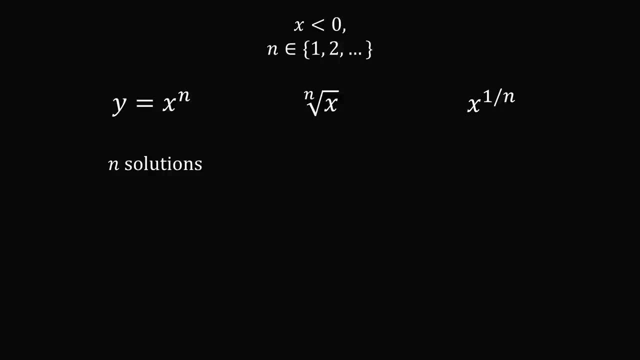 So y is equal to x, to the power of n. Of course we'll have n solutions here. Now the nth root of x, somewhat will depend on context. There are reasons to use the real root value. So let's say, for some reason you had a negative velocity. 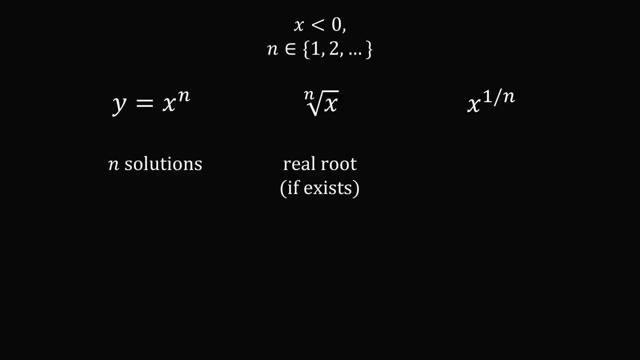 and you need to take the cube root of that. You're working on a physics problem. Well, it might make sense to take the real root, because you want this real value for your solution, But this could also refer to the principal root, which may sometimes be a complex number. 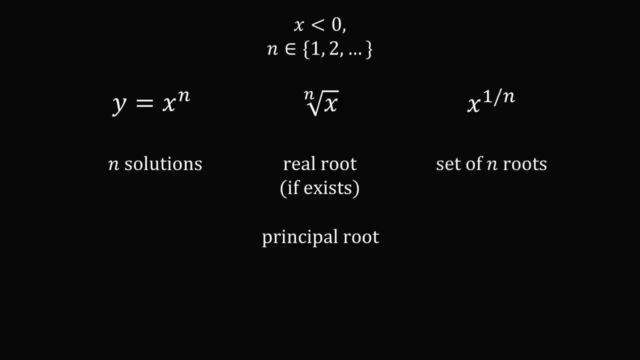 Now, x to the power of 1 over n can be used to denote the set of n roots, but it might also be used to denote the principal root. This will depend a little bit on context, But the general point is that the nth root of x and x to the power of 1 over n may not be the same thing. 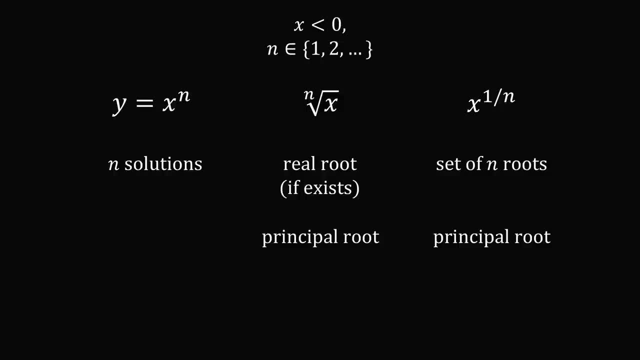 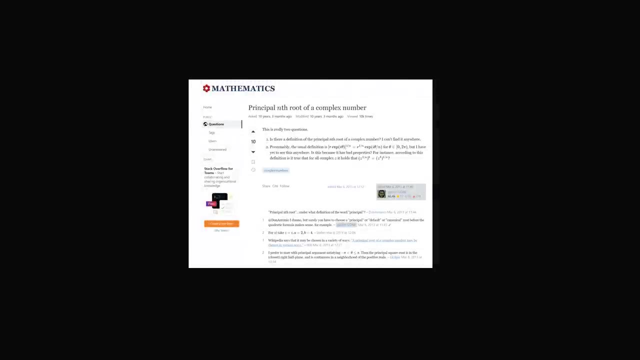 in all contexts, and it's an important distinction to know. The definitions and conventions presented in this video are what I found in my textbooks and in my research online, But I will warn that there is no standard definition of a principal value that's accepted across all texts. 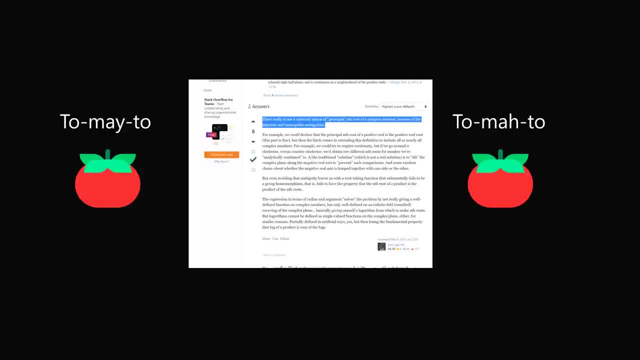 But just because one text says one thing and another text says another thing doesn't mean you have to call the whole thing off. Just pay extra attention to the convention that's being used, and then you can readily solve the problem and be on your way. 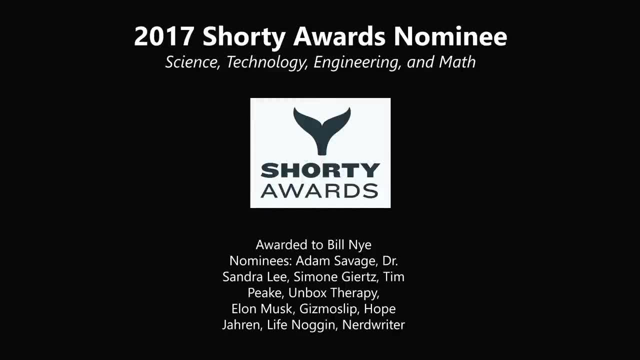 Thanks for making us one of the best communities on YouTube. See you next episode of Mind Your Decisions, where we solve the world's problems one video at a time.